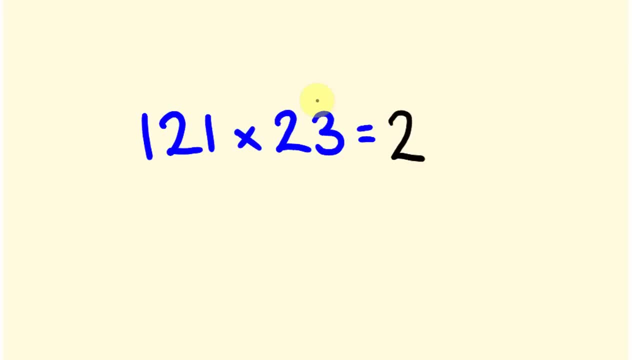 Okay, so we get our 2.. Then what we're going to have is two middle digits, which we're going to come back to in a little bit. I'll show you how to work these out, But we're going to go straight to working out our last digit. The way that we work this out is multiplying the last digits here. So 1 times 3 is 3.. 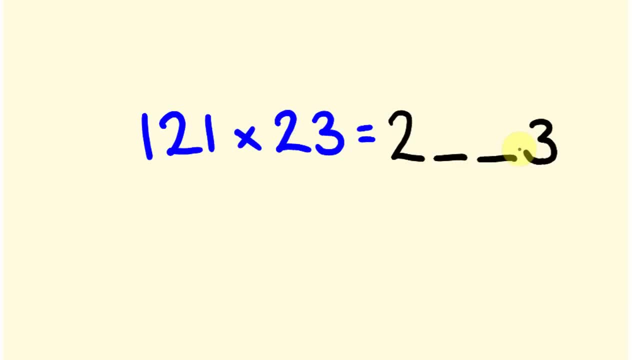 Now let's have a look at this Now. so far, this is much like this other method of multiplication where we had a look at where we're multiplying two and two digit numbers together, But this is a slight tweak on it. Now, what we do now is we're going to work out this particular number here. 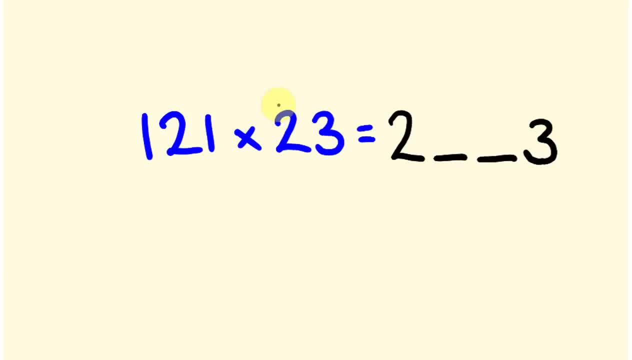 What we do is we do this thing called rainbow multiplication. We're going to multiply this number by this number and this number by this number. You can see why we call it rainbow multiplication. yeah, And we're going to add our answers together. It will give us the number that's going to go in here. 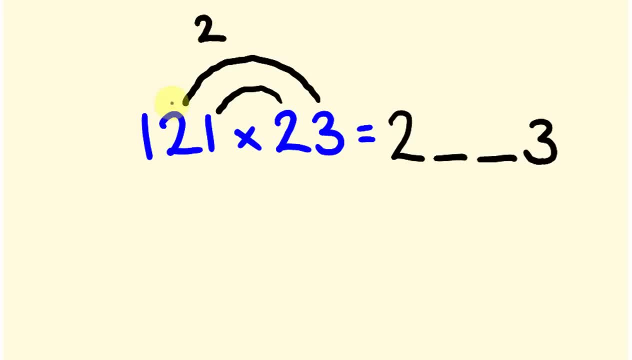 Okay, so 1 times 2 is 2, and 2 times 3 is 6.. We're going to add these answers together to get an 8.. Okay, so 8 is going to go in here. All right, to get this number here, the next part of our answer. we're going to do this rainbow multiplication. 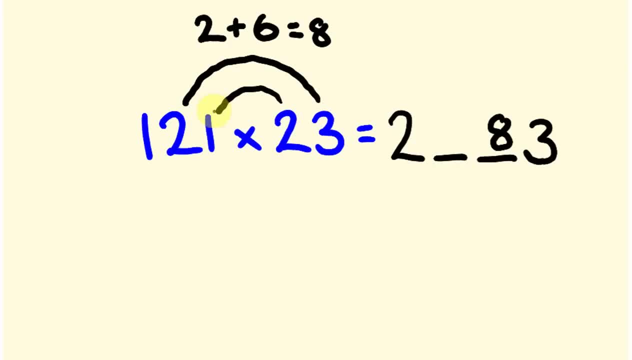 I'm going to do it underneath here, but I'm going to move these parts across one, So 2 times 2 and 3.. 3 times 1, okay, So 2 times 2 is 4.. We're going to add that to 3 times 1,, which is 3.. 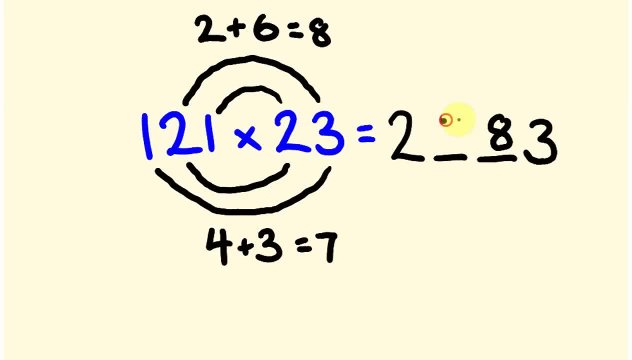 So 3 plus 4 equals 7.. So our answer is 2,783,, which is the correct answer. So that's a really really cool method. yeah, It's not too confusing. I don't think there's any bit there that you won't be able to remember. 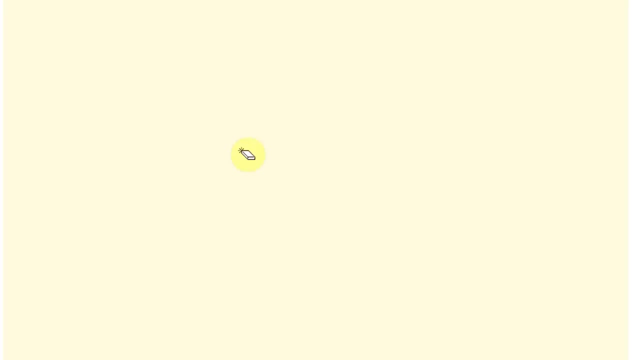 But hey, let's see, I'll tell you what I'll go through. one more example. Then I'll give you a bunch of ones. Do it for yourself and see how you go with it. In fact, I'm going to leave some of the harder ones, I think, for you okay. 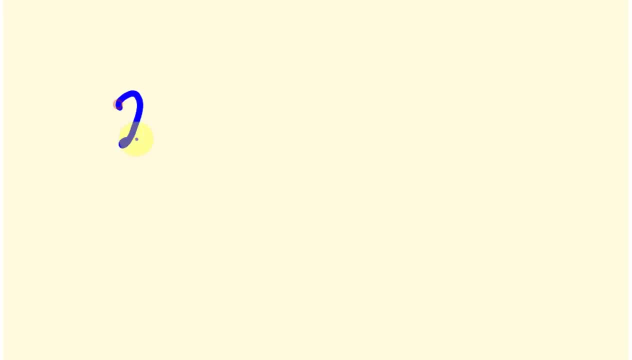 What about we go through one more of these 242. And we multiply this by 32.. Okay, So to get this first part of our answer, what do we do? We multiply these 3 times 2 is 6.. 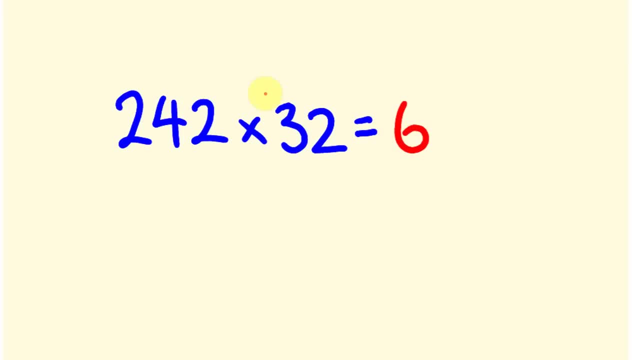 Okay, I'm going to put this in a red pen. So 6.. Okay, 2, threes is 6.. We leave two spaces, 1, 2.. Okay, Then what we do is we get the last part of our answer, 2 times 2,, which was 4.. 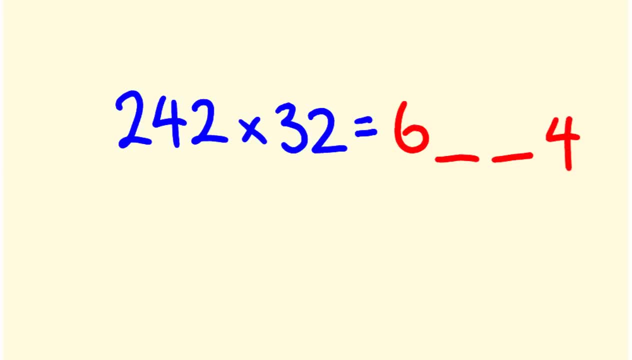 Okay, So we're doing pretty well so far, you're right. Okay, let's get this digit here. So what we did is we do this rainbow multiplication thing. yeah, This is 3 times 2. And we're going to add that to 2 times 4.. 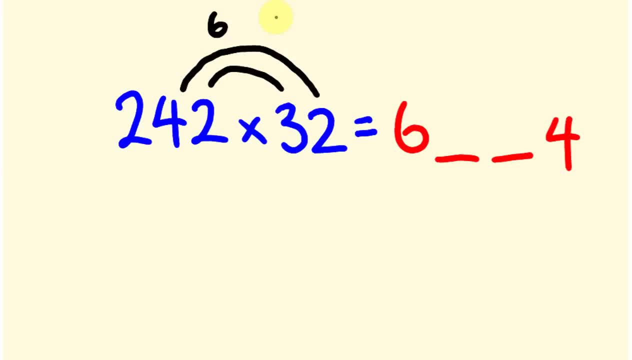 So 3 times 2 is 6.. And we're going to add that to 2 times 4, which is 8.. So 6 plus 3. 8 equals 14.. Now I'm going to put the 4 down in here. 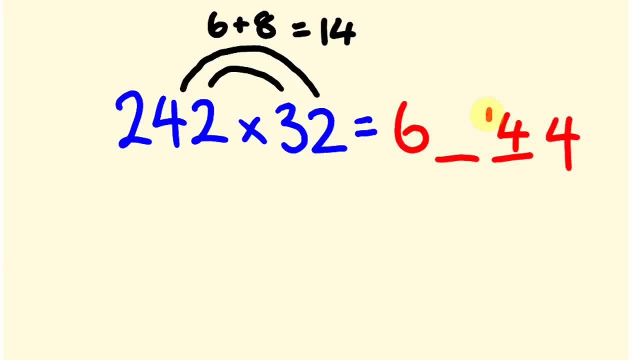 But what I'm going to do is I'm going to put the 1 there, because we're going to be carrying that into our next part of our answer here. So the 14, we only put the 4 part of it down and we're going to put the 1 just there, just. 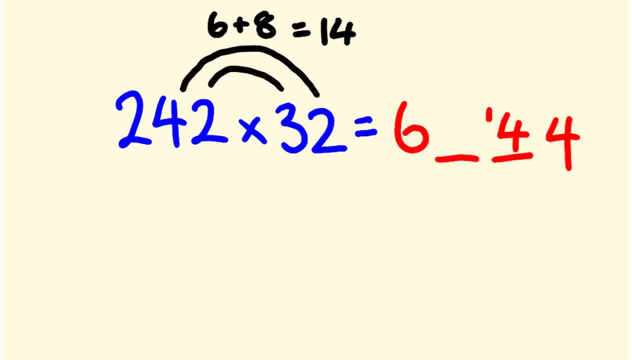 to remind us that we're going to be putting it into here. So let's do the next part of our rainbow multiplication: 3 times 4, which is 12.. We're going to be adding to 2 times 2,, which is 4.. 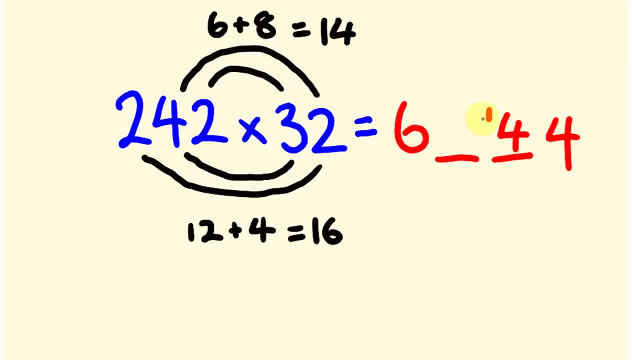 So we add those, we get 16.. 16 plus 1: here we get the answer of 17.. So that's going to become a 7. And I'm going to have to move this 1 across into here. 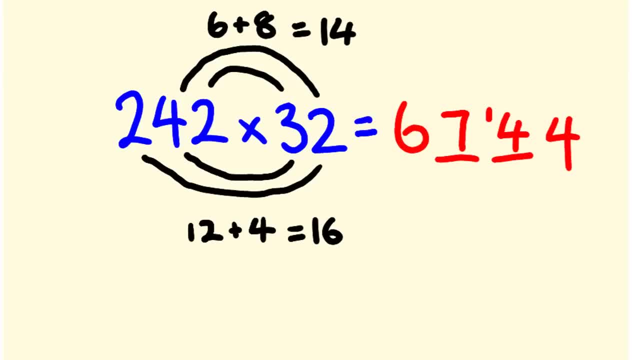 So what are we going to do? We are going to add it to the 6 here, So the 6 is going to become a 7, okay, Well, we added that 1 in, So our answer is 7,744.. 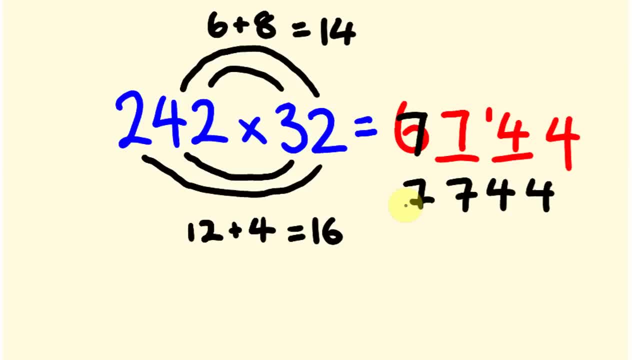 Okay, So hopefully that worked out for you. Okay, What about I give you a couple of hard examples? These are the ones. hey, these aren't that hard. okay, It's the same exact same method, As long as you can remember where you have to, you know, place things and carry things. 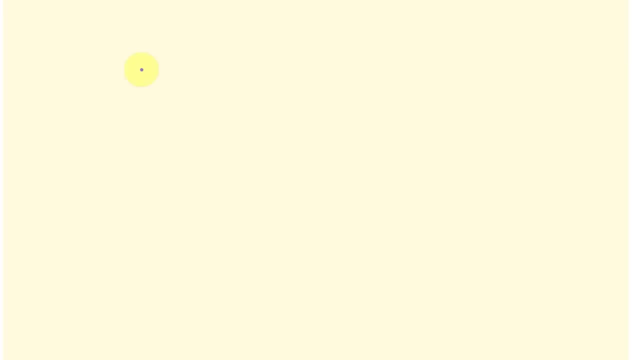 and that sort of deal, you'll be pretty right. So I'll give you a nice easy one to start off with. then I'll give you the hard one, Okay, So what about 122 times 32?? That will be the first one I'll get you to do. 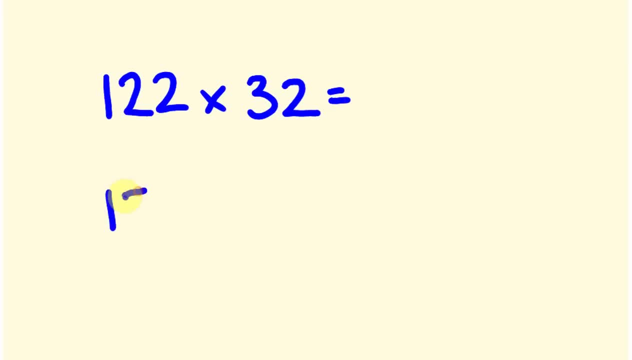 And then I'm going to get you to do 122.. And then I'm going to get you to do 153.. And we're going to multiply that by 61.. Okay, Pause the video. give them a go and I'll see you back here in a minute. 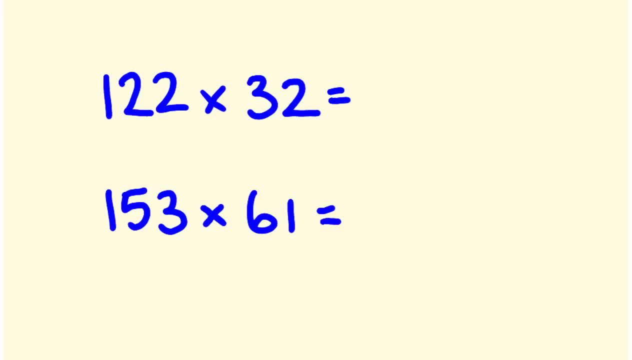 Okay, Hopefully you've done those and let's check how you went on those. So okay, 1 times 3 is 3.. Two spaces boom and boom and 2 times 3,. 2 times 2 is 4, okay. 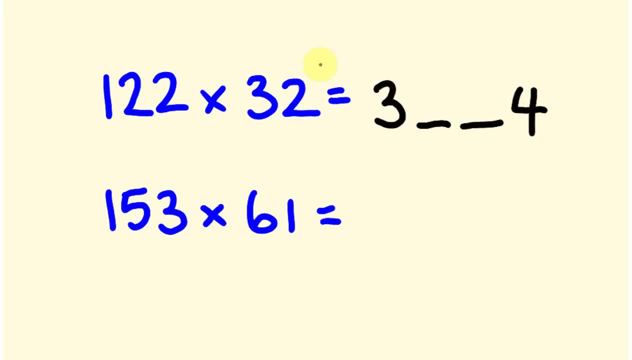 So we're doing pretty well so far. Hopefully you're pretty good so far. Now, what we do is we do this rainbow multiplication, So we're going to be getting 6 and adding this to 4, which is 10.. 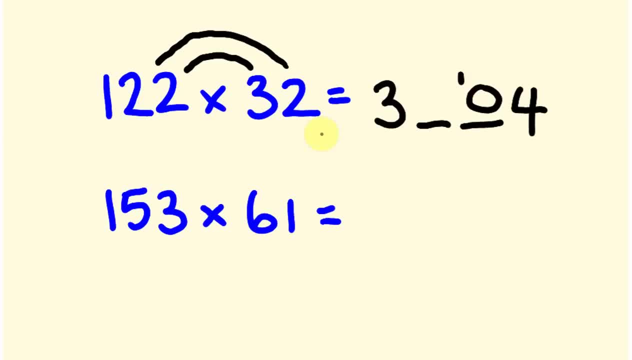 So I'm going to put a 0 there and a 1 there. We're going to be putting it here. We're going to go 3 times 2, which is 6.. To that we're going to add 2.. 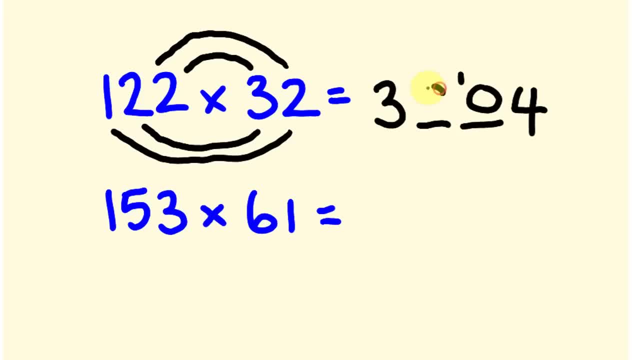 6 and 2 is 8, plus this 1 here is 9.. So did you get the answer to 3,904?? If you did, congratulations. If you didn't, well, you can just have a quick look over how I did it there and see where you made your mistake. 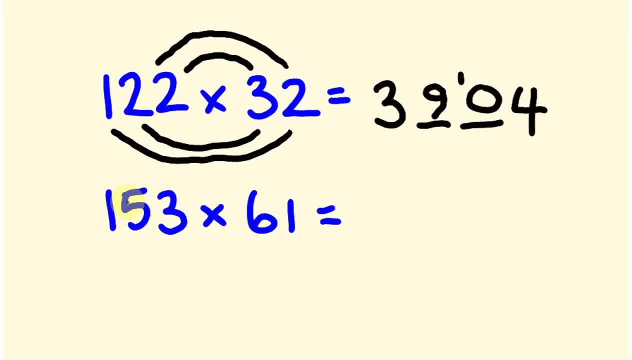 Fix it up, okay. Okay, let's go to this last one here. So 1 times 6 is 6, couple of spaces. 1 times 3 is a 3, okay, Now let's do this rainbow multiplication here, okay. 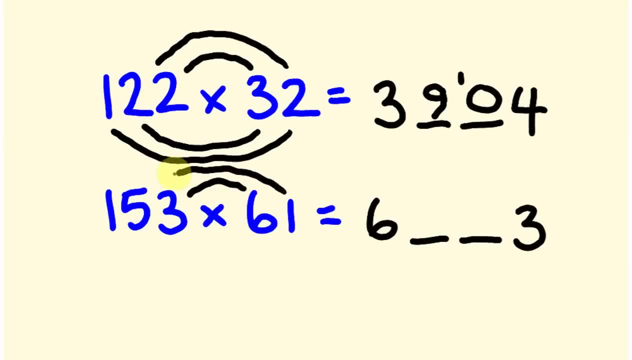 So we're going to go 3 times 6,, which is 18,, and 1 times 5,, which is 5,. 18 plus 5 is 23,. okay, So we'll put the 3 there and I'm going to put my little 2 up there. 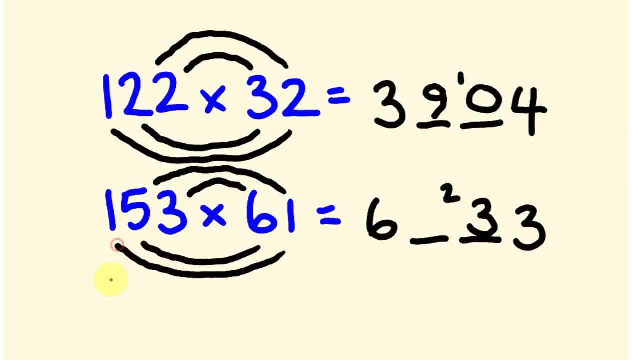 6 times 5 is 30,, 31, plus 2 is 33.. So that 3 is going there and another 3 is going to have to be added to our 6 here. So this is going to become a 9.. 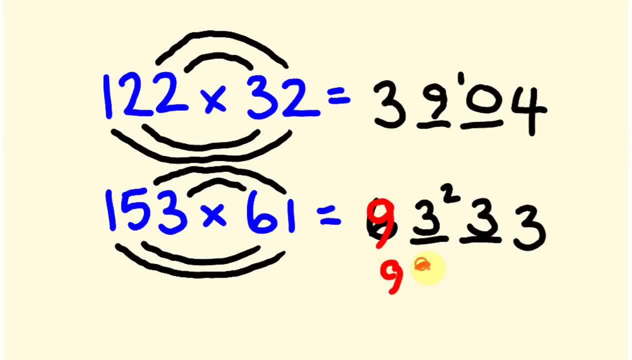 Okay, so our answer is 9,333.. So hopefully you really really get the hang of that method. It's not a bad method, eh? Tell us what you think about it, Tell your friends, Show everybody, All right. Anyway, thanks for watching. See you next time, Bye.